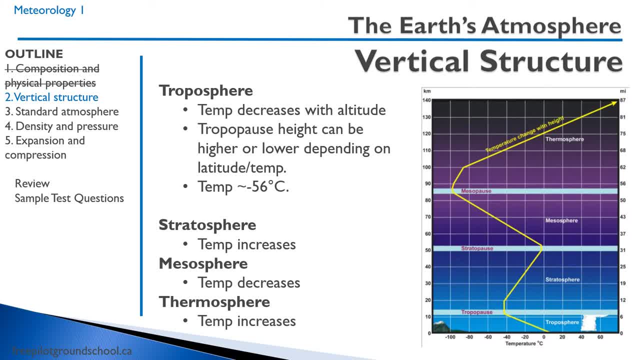 into different vertical structures. The first structure that we'll talk about is the troposphere. The troposphere is where the majority of the weather that we're dealing with occurs. It's from about the surface to about, let's say, 35 to 40,000 feet, depends on the latitude. 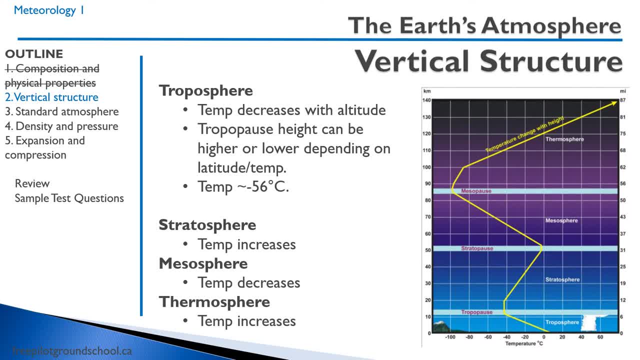 depends on the temperature In the troposphere. the temperature decreases with altitude. The height of the tropopause- so the tropopause is the end of the troposphere- can be higher or lower depending on the latitude or temperature. I've seen up in the arctic cold winter. 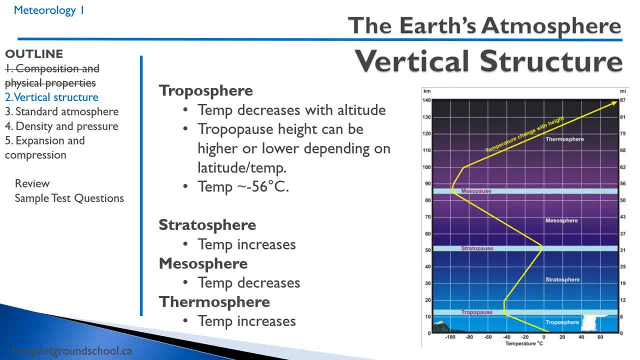 cold winter night. the height of the troposphere is very low, like 8,000 feet, something like that. The temperature at the top of the troposphere always ends up being about minus 56 degrees Celsius. The next layer is the stratosphere. Within the stratosphere the temperature starts. 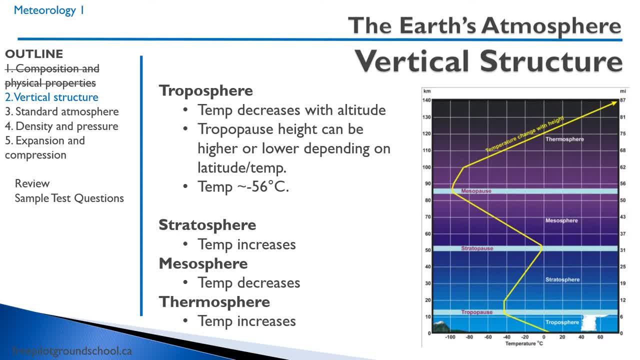 increasing slightly, reaching approximately freezing at the stratopause. Above the stratosphere is the mesosphere, or mesosphere. In here the temperature again drops drastically. Above the mesosphere is the thermosphere, which point the temperature increases considerably with height. It's at this point of energy. 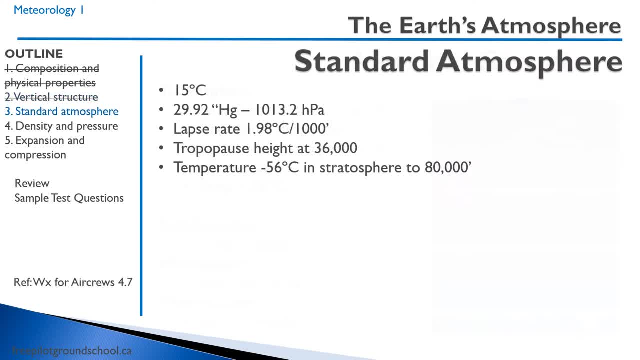 you end up in space. Let's talk about the standard atmosphere. The standard atmosphere is basically the average atmospheric properties across the world, and these numbers will come up often in your meteorological training. First off, the standard atmospheric temperature is 15 degrees Celsius. The standard pressure is: 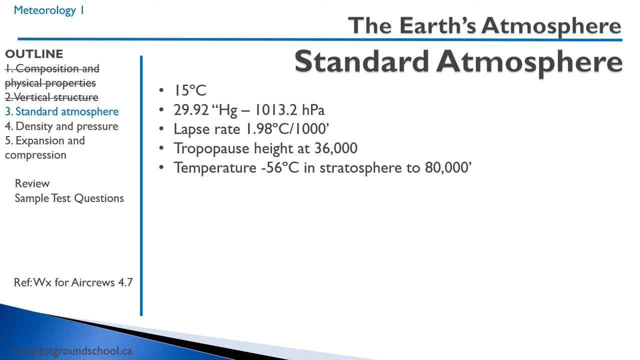 29.92 inches of mercury- that's the altimeter setting- or 1,013.2 hectopascals. The lapse rate, that is the change of temperature with altitude, is 1.98 degrees Celsius per thousand feet and the standard triple cos height is: 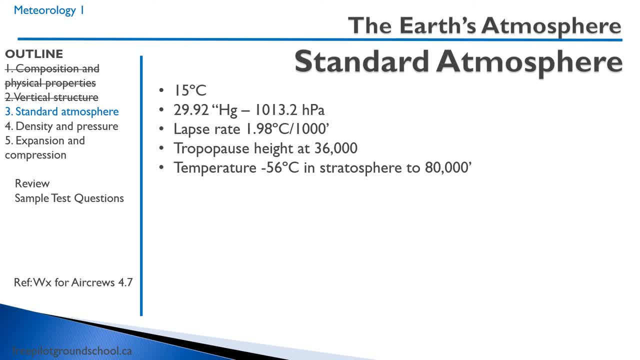 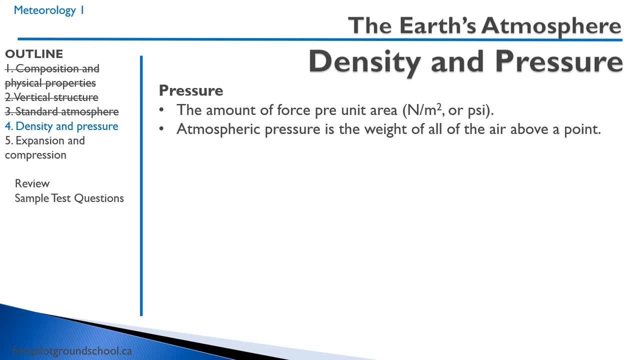 36,000 feet, Temperature is minus 56 degrees Celsius in the stratosphere. to 80,000 feet, Pressure is the amount of force per unit area, so, for example, newtons per meter squared, which is called a Pascal, Also a pound per square inch, pound being force and square inch. 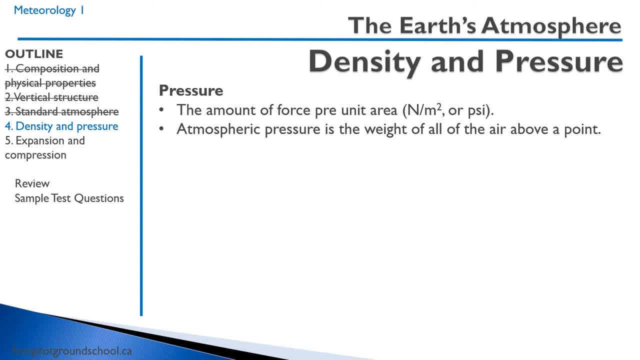 being the unit area, The atmospheric pressure is the weight of all of the air above a point. Let's just say we're flying a 10,000 feet and we measure the atmospheric pressure at that point that we have a column, let's say a one square inch column. 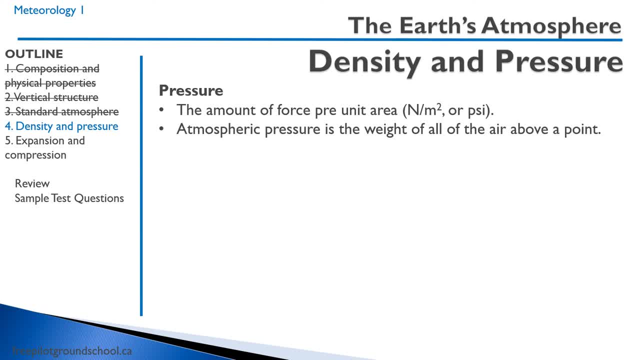 above the atmosphere. that point, That would be our atmospheric pressure. Density, on the other hand, is the mass of the air per unit volume, such as kilograms per cubic meter. Warmer air is less dense than cold air and therefore will rise This topic, that of atmospheric expansion. 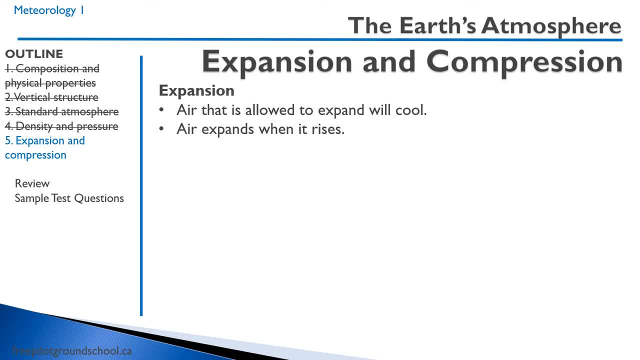 and compression will come up frequently in your meteorology lesson, especially when we talk about unstable air Expansion. when air is allowed to expand, it will cool and air expands when it rises. Conversely, air that is compressed heats up. Air compresses when it subsides or 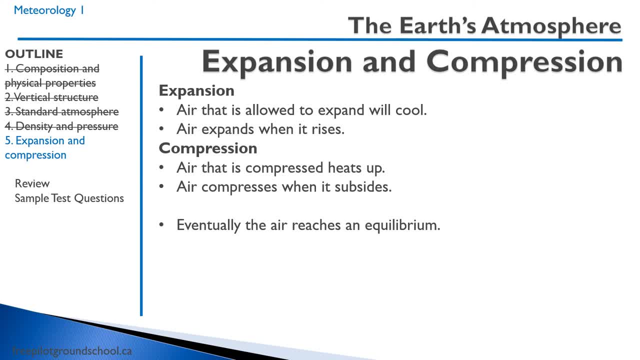 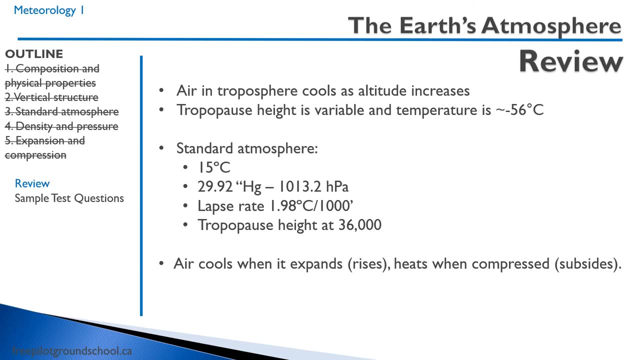 moves down Eventually, the air reaches an equilibrium at a certain point, and this will become evident when we're discussing stability of the air and thunderstorms. Air in troposphere cools as altitude increases, The tropopause height is variable and the temperature is minus 56 degrees Celsius. The standard atmosphere is 15 degrees Celsius. 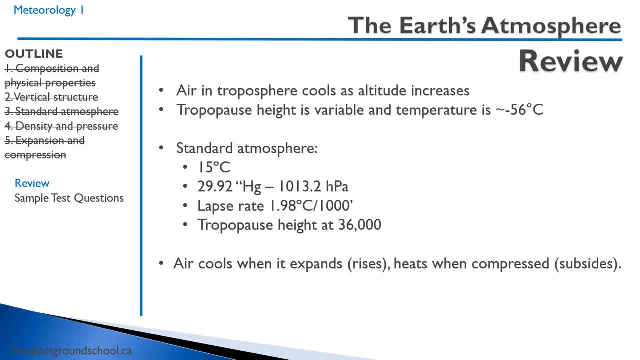 29.92 inches of Mercury, 1-1,013.2 hPa, a lapse rate of 1.8 degrees Celsius per thousand feet and a tropopause height of 36,000 feet. Air cools when it expands or rises and heats. 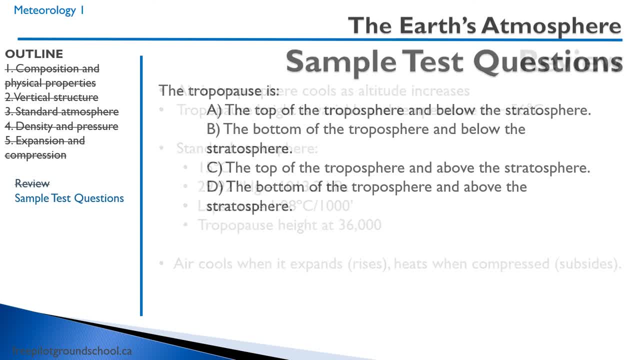 up when compressed Air's temperature is minus 2850 to 10 to 200 degrees Celsius when cruise or subsides. Let's work our way through a few sample test questions. The tropopause is A the top of the troposphere and below the stratosphere, So that's correct. Let's keep. 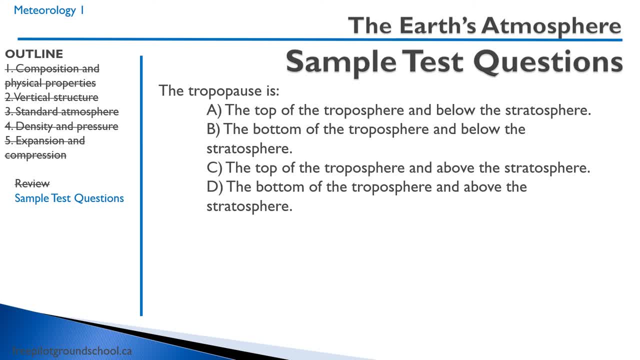 reading B: the bottom of the troposphere and below the stratosphere. No, that makes no sense, because the bottom of the troposphere- that would be well the Earth- is at the bottom of the troposphere. C: the top of the troposphere and above the stratosphere. No, that's not correct.